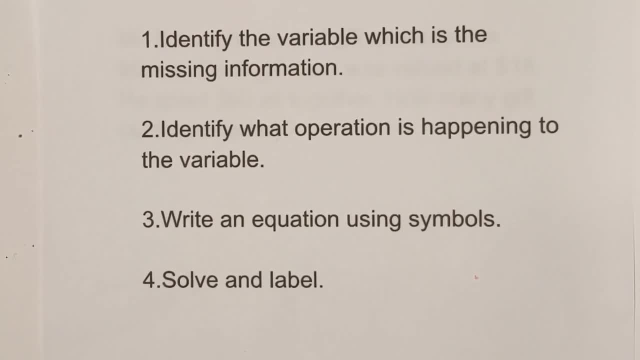 about solving this, and this works pretty well. First you need to identify the variable, which is the missing information, In other words, what are they asking for? Then you identify what operation is happening to the variable. Now there are a couple words that kind of give you. 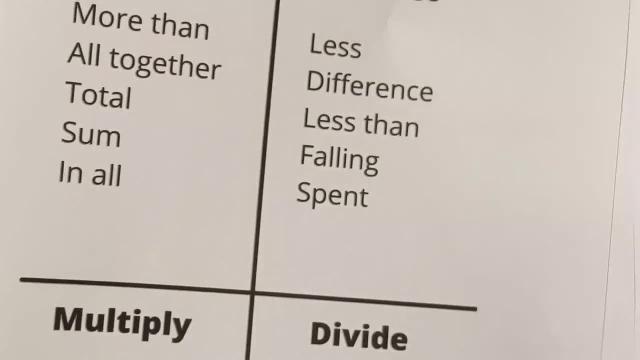 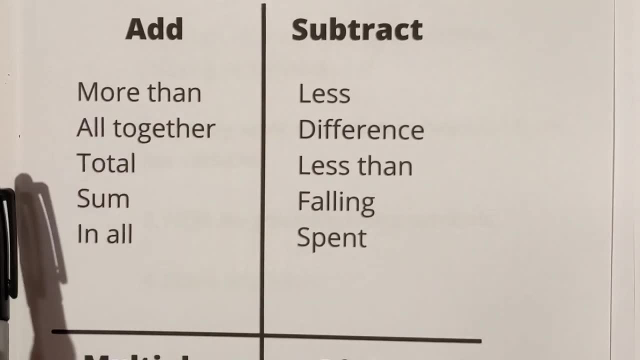 clues, and I'll show you these. For addition, you'll sometimes see more than altogether total sum all in, And for subtraction you'll see less difference, less than falling or spent. And then for multiplication, 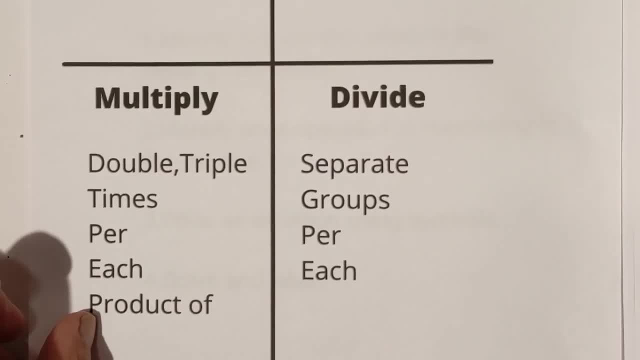 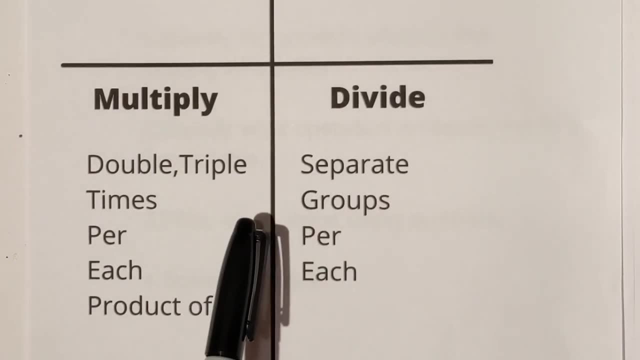 move this up, you'll see double, triple times per each or a product of And for division, separate groups, and then per and each. And, yes, per and each are used on both of them. You just have to. 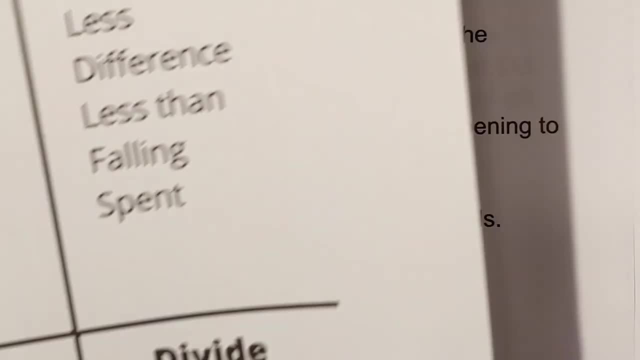 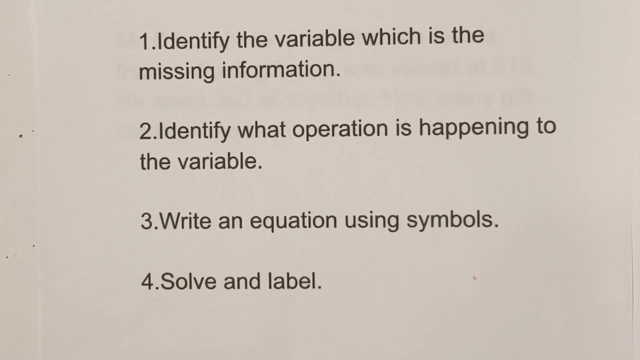 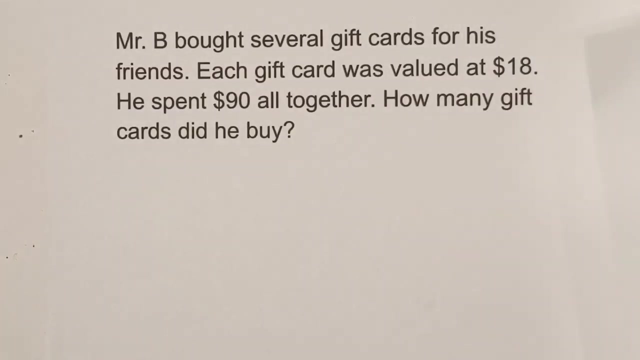 read the content. So let's apply these steps right, And then, after you do this, you then write an equation using symbols and then you solve and label. So let's try to use these steps on a couple example problems And see if we can figure this out. So let's get started, Okay, So problem one is the one we just 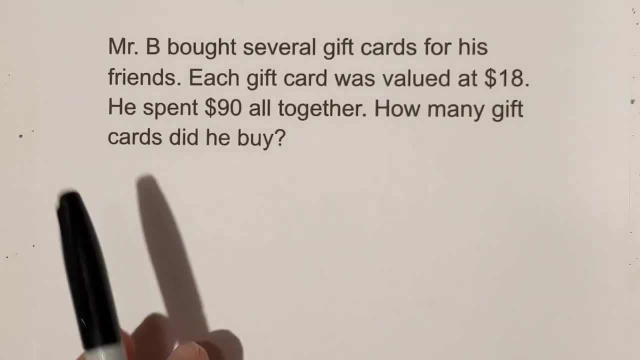 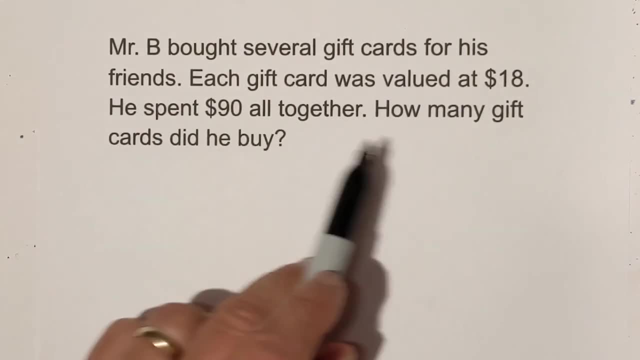 read: Okay, So Mr B has been generous and he's bought some gift cards for his friends. Okay, And it says each gift card was valued $18.. He spent $90 altogether. How many gift cards did he buy? 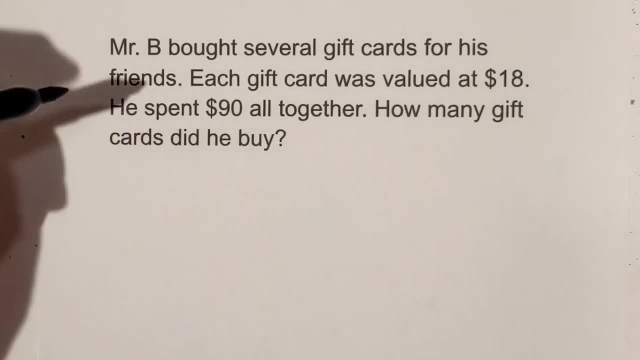 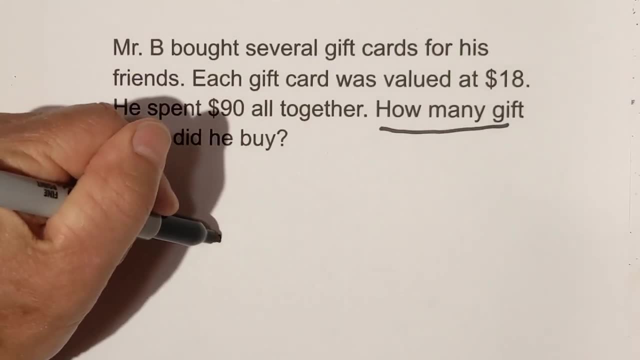 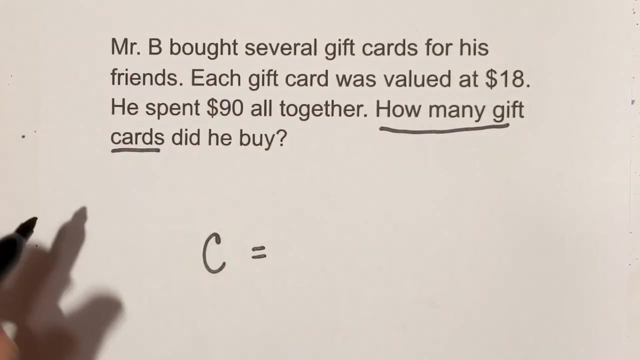 So let's identify the variable It is. what is the missing information? He wants to know how many gift cards, Okay. So why don't we go with a C for cards, Okay? Next, he knows that he spent $90 altogether. Altogether is one of the. 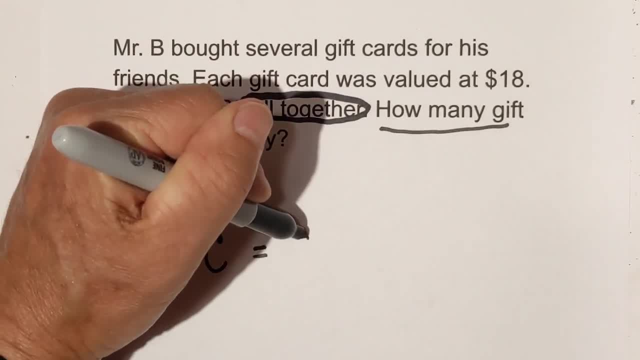 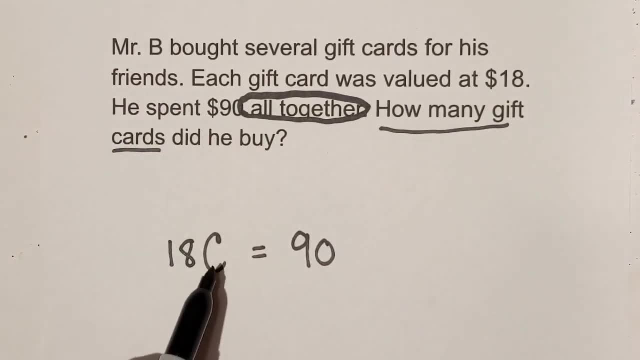 multiplication words, And so altogether is the total. So we'll go 90 for the total. And we know that he spent $18 times the variable to equal 90. And the variable is the number of gift cards. So now all we do. 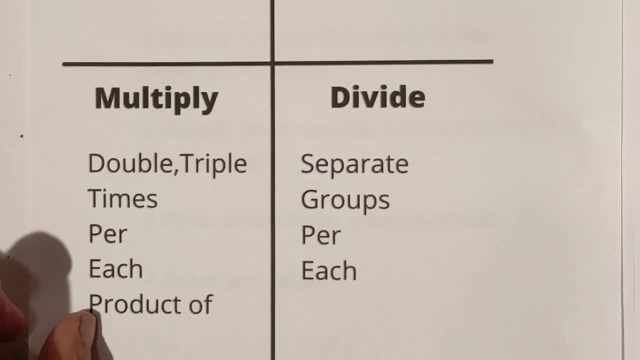 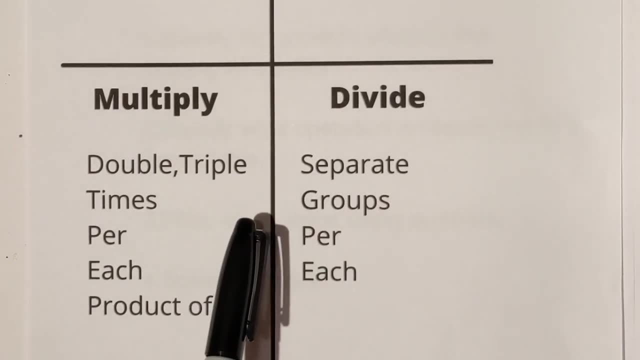 move this up, you'll see double, triple times per each or a product of And for division, separate groups, and then per and each. And, yes, per and each are used on both of them. You just have to. 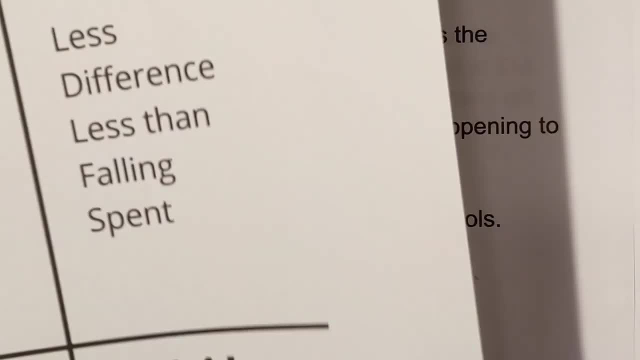 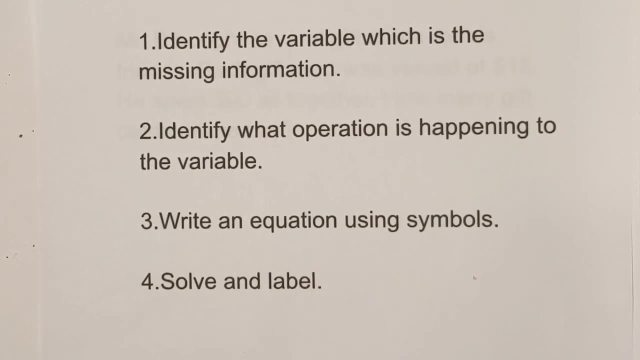 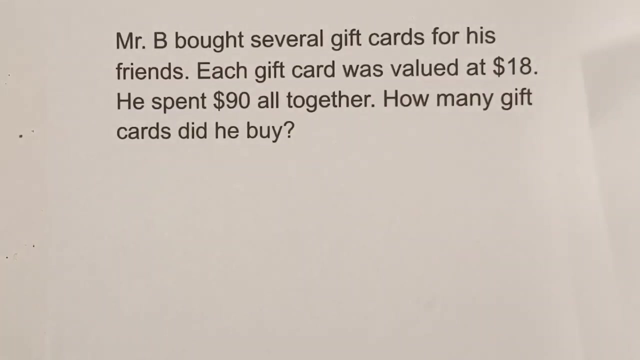 read the content. So let's apply these steps And then, after you do this, you then write an equation using symbols and then you solve and label. So let's try to use these steps on a couple example problems, Uh, and see if we can figure this out. So let's get started, Okay. So problem one is the one we 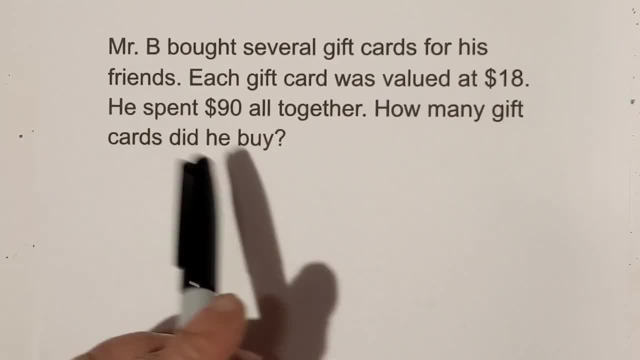 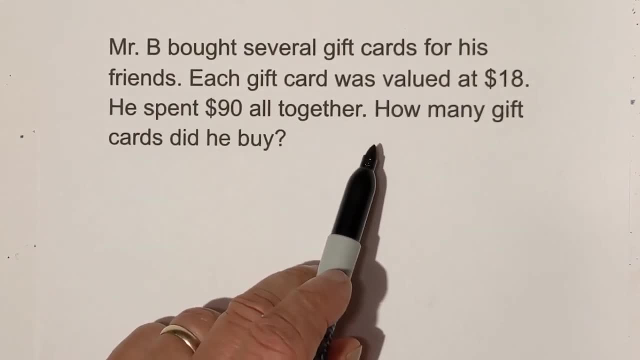 just read: Okay, So Mr B has been generous and he's bought some gift cards for his friends. Okay, And it says each gift card was valued $18.. He spent $90 altogether. How many gift cards did he buy? So let's identify the variable It is. what is the missing information He wants to know? 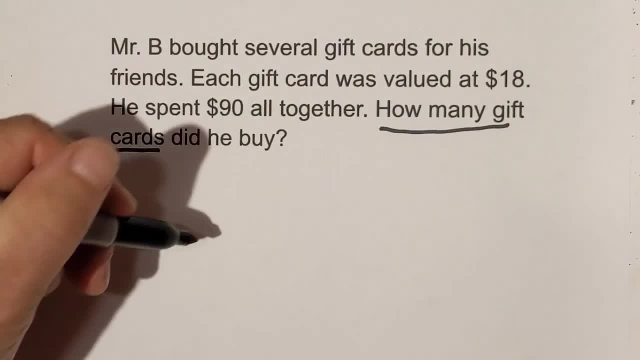 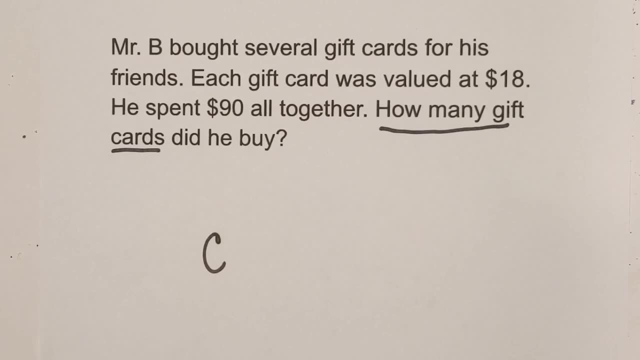 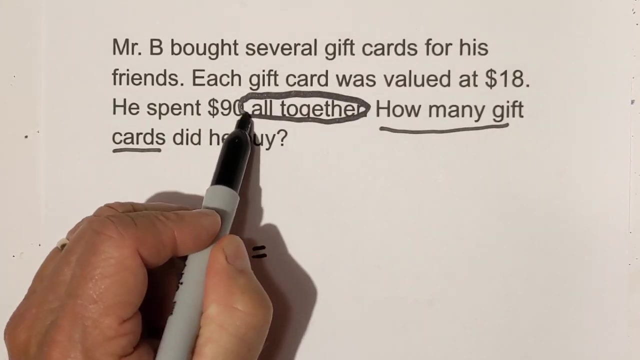 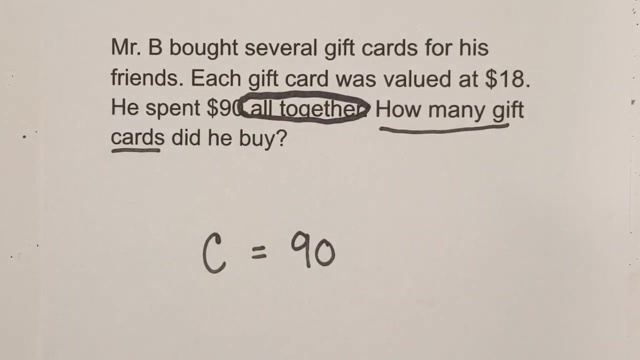 how many gift cards, Okay. So why don't we go with uh C for cards? Okay. Next, he knows that, uh, he spent $90 altogether. Altogether is one of the multiplication words, And so altogether is the total. So we'll go 90 for the total, and we know. 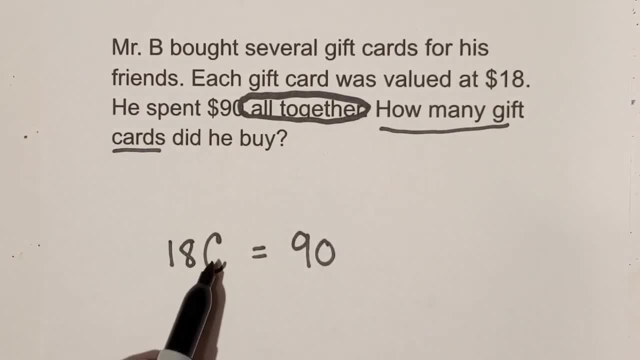 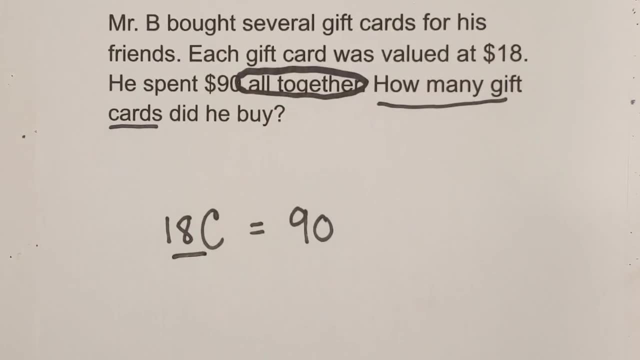 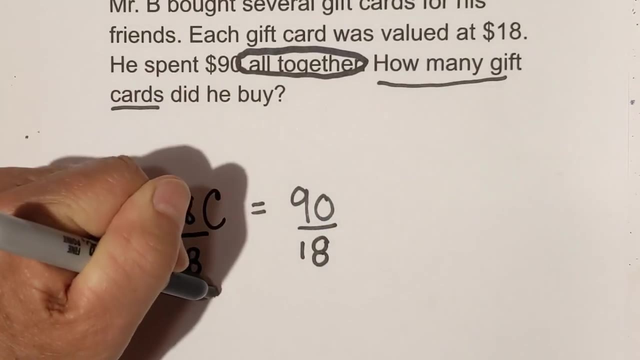 that he spent $18 times the variable, to equal 90. And the variable is the number of gift cards. So now all we do is, let me make sure, Let me move this up just a little bit- We divide each side by 18.. Okay, Uh, bring down the C. 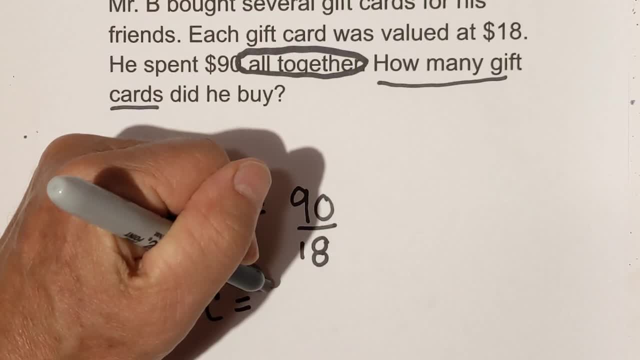 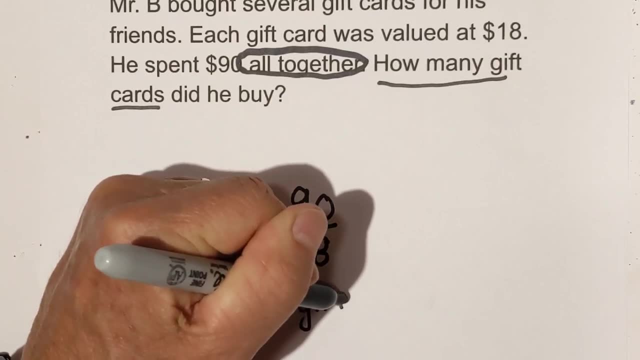 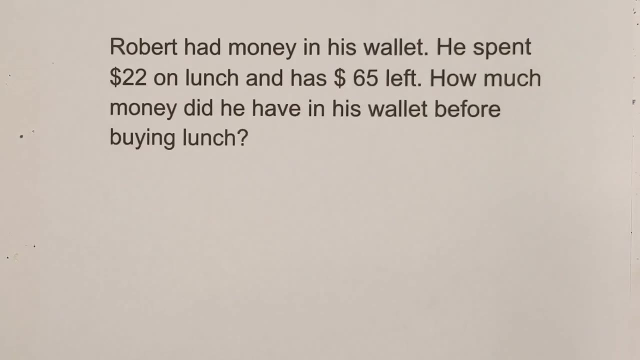 equals and 90 divided by 18 is five. So we've solved it and now we need to label it. It was five gift cards. Okay, That's the first one. Let's look at a couple more examples. Okay, Robert had money in his wallet. He spent $22 on lunch and has 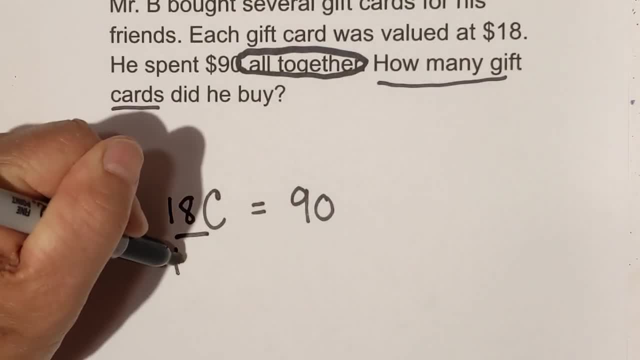 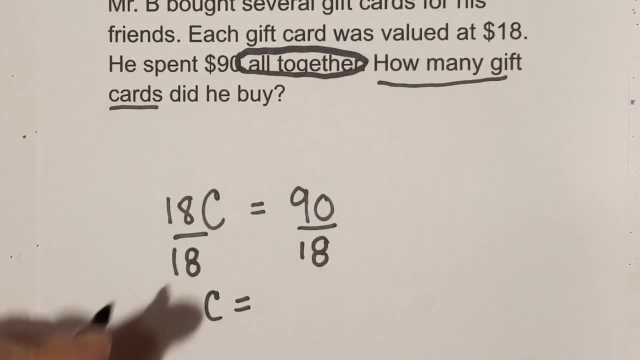 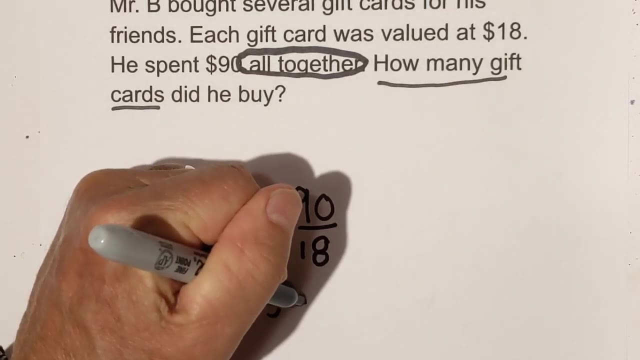 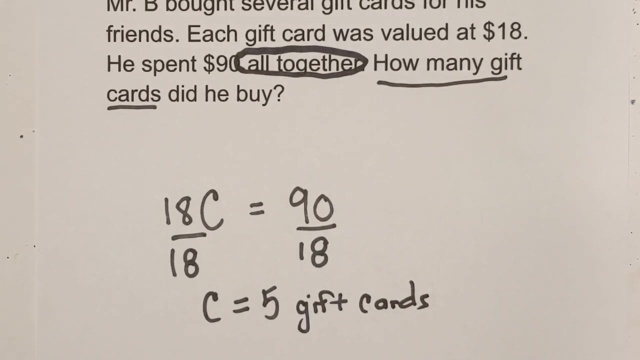 is. let me make sure, move this up just a little bit. we divide each side by 18. okay, bring down the c equals and 90 divided by 18 is 5. so we've solved it and now we need to label it. it was five gift cards, okay, that's the first one. let's look at a couple more examples. 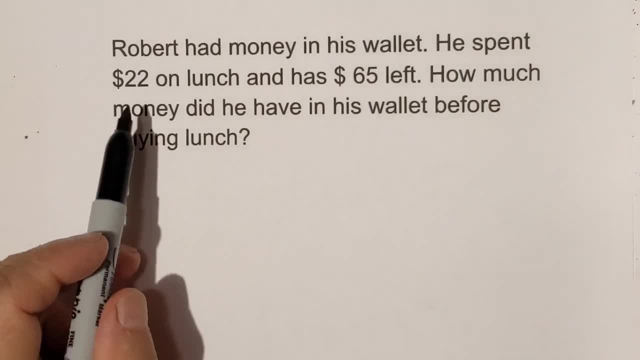 okay, Robert had money in his wallet. he spent $22 on lunch and has $65 left. how much money did he have in his wallet before buying lunch? okay, so first let's identify what the variable is, and we want to know how much money he had in his wallet before lunch. so why don't we call that m for money? 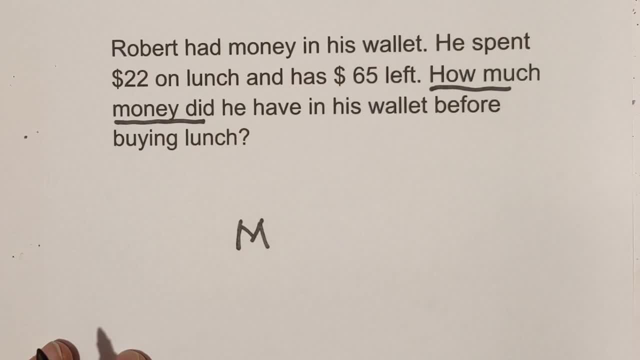 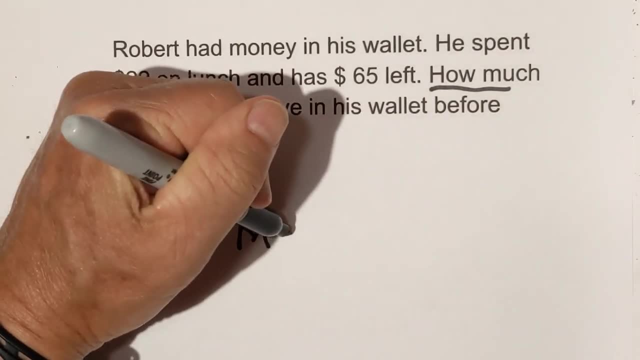 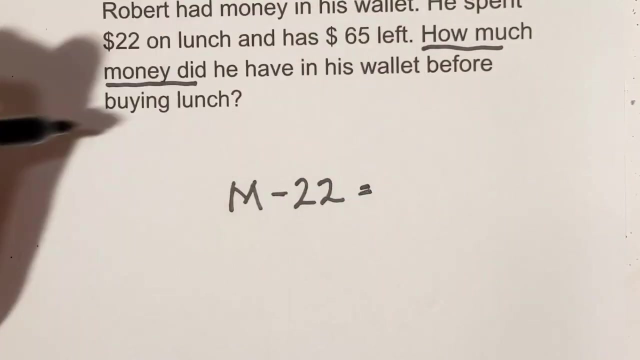 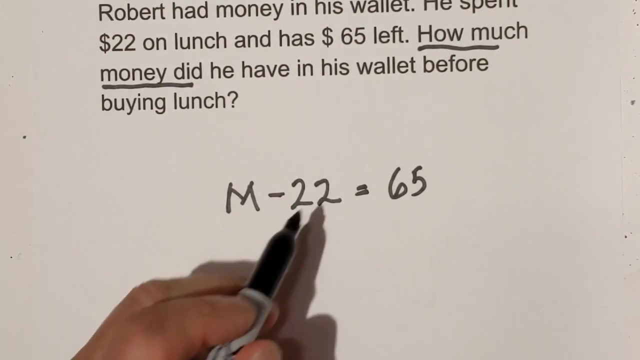 okay. next, we know that um, he spent money, um and m is the total, so he subtracted $22 on lunch and that's going to equal our total of what we have left, which is 65. so now we have the variable and we have the operation. okay. 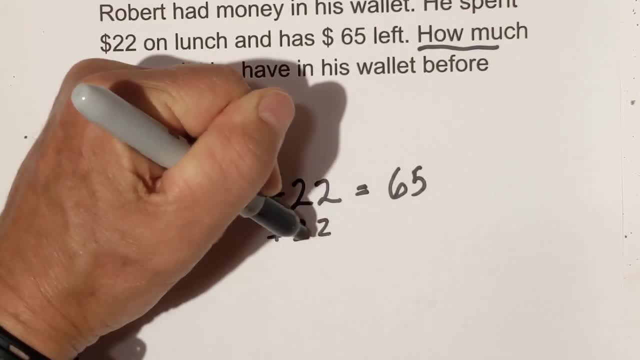 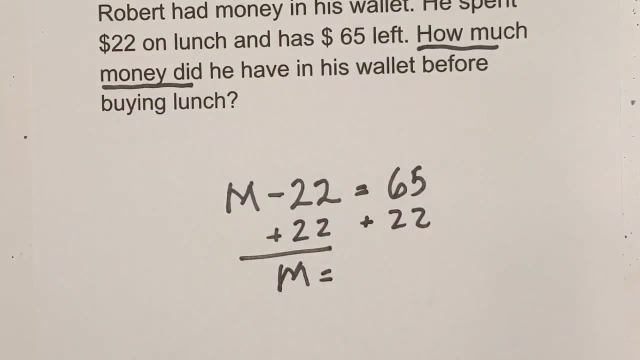 now all we do is solve. in order to solve this, we go 22 on both sides, we add 22, both sides, bring down the m and that equals 65 plus 22 is 86. okay, so now we have the variable and we have the operation. okay, now all we do is solve in order to: 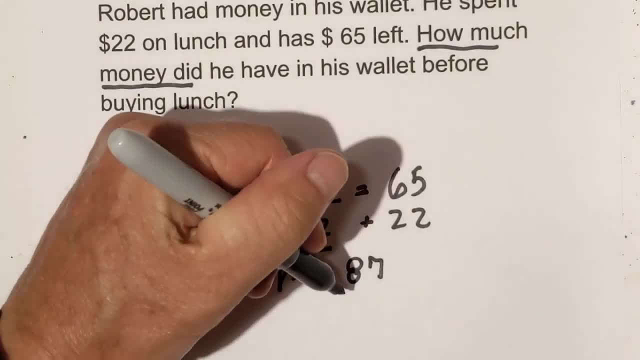 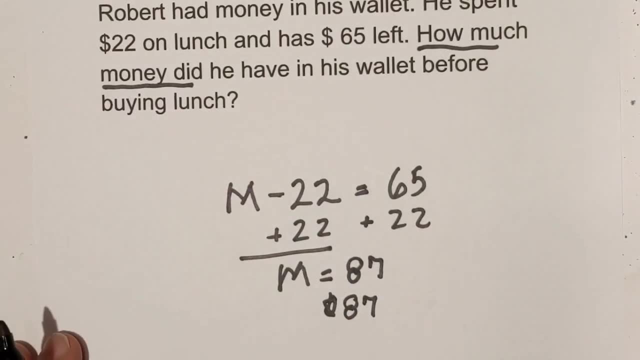 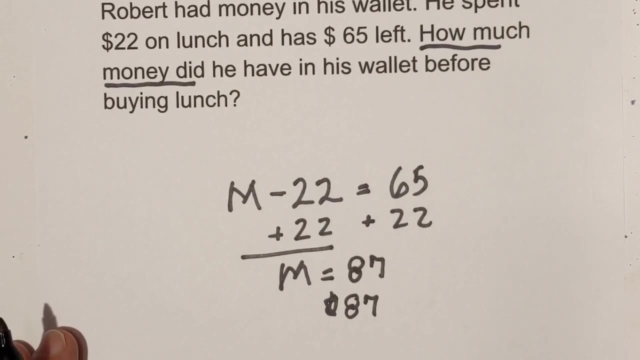 solve it. so now we have solved it and now we need to label it, and that is $87. so he started with. that's a terrible dollar sign. by the way. he started with $87, he spent 22 and now has $65 left in his wallet. one more, okay. Bob makes cupcakes to sell at his store. he sold 240. 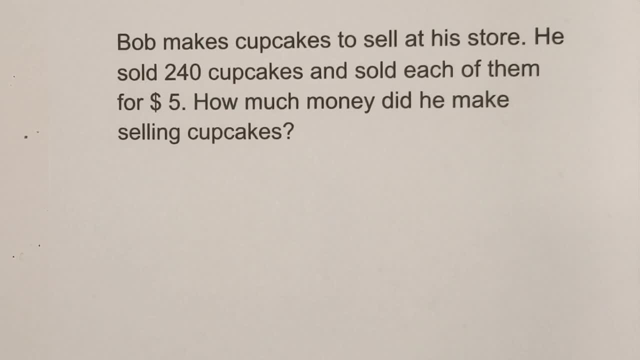 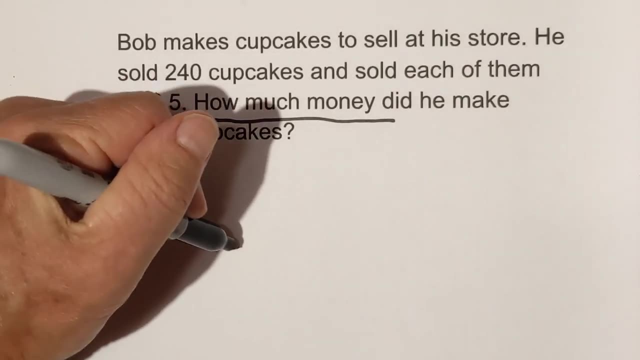 cupcakes and sold each for five dollars. how much money did he make selling cupcakes? okay, the variable is m and m is the total. so now we have the variable and we have the operation. okay, now all we do is solve in order to: how much money did he make? so let's go with again, we can go with m for money. okay, I'm going to move. 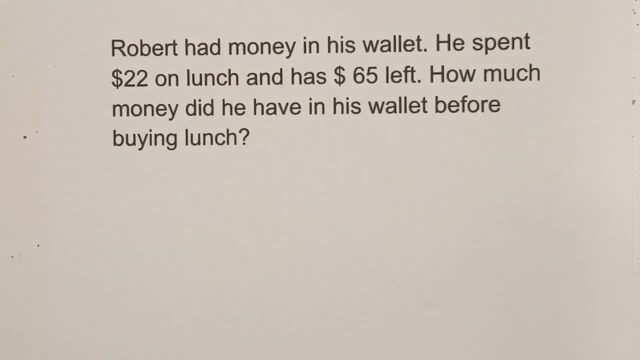 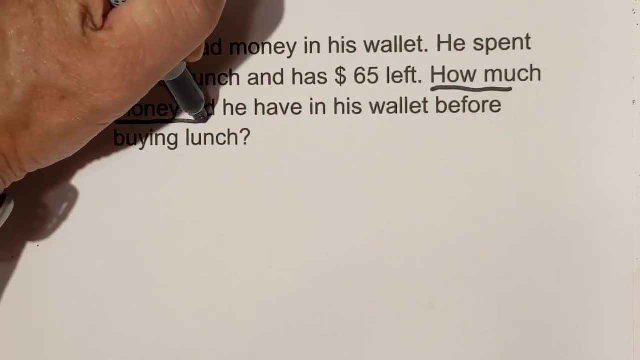 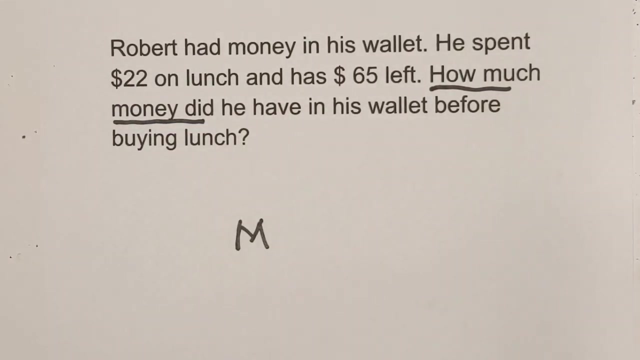 $65 left. How much money did he have in his wallet before buying lunch? Okay, So first let's identify what the variable is, and we want to know how much money he had in his wallet before lunch. So why don't we call that M for money, Okay? Next we know that, um, he spent money. 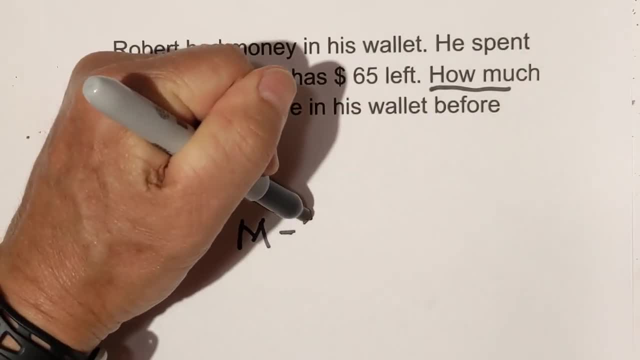 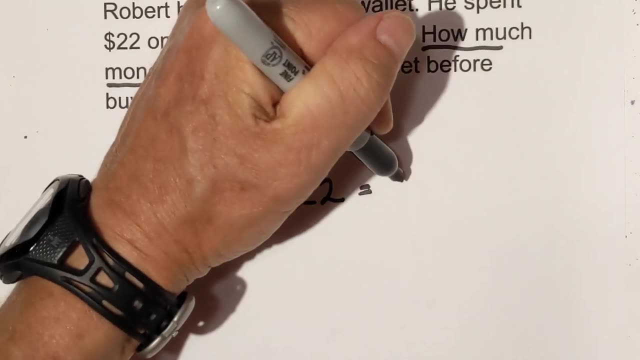 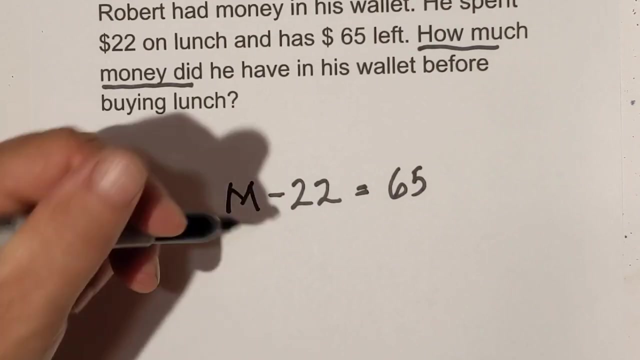 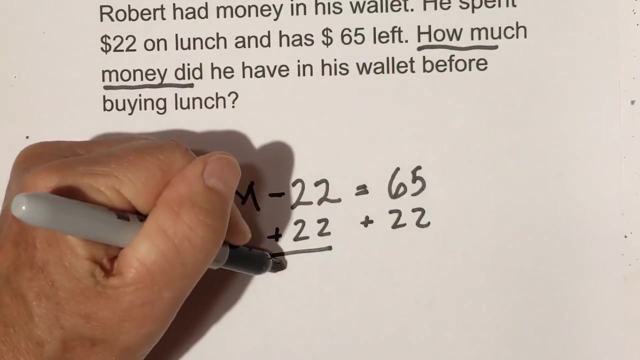 and M is the total. So he subtracted $22.. Okay, So now we have the variable and we have the operation. Okay, Now all we do is solve. In order to solve this, we go 22 on both sides, We add 22 both sides, Bring down the M and that. 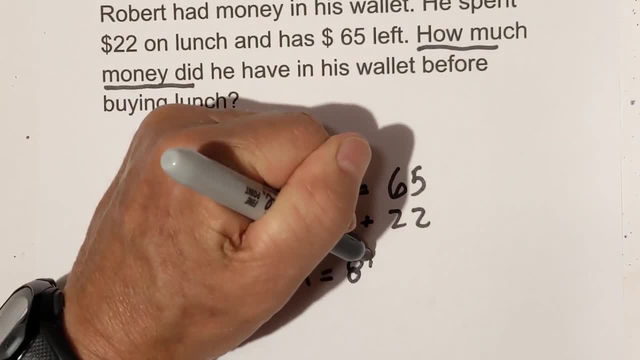 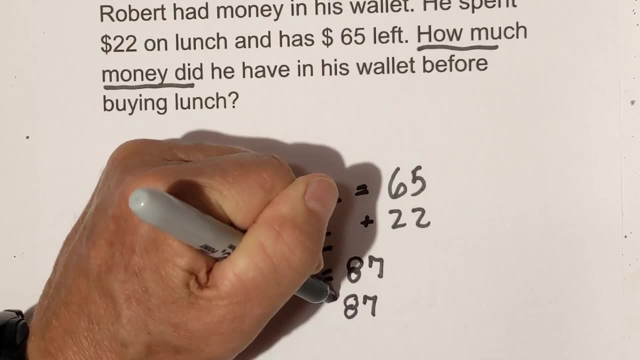 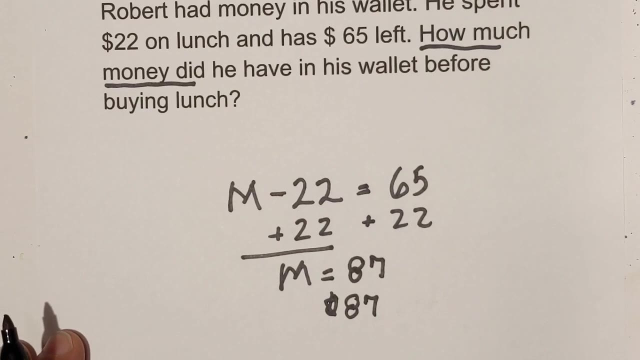 equals 65 plus 22 is 87. So now we have solved it and now we need to label it, and that is 87. So he started with. that's a terrible dollar sign. by the way, He started with $87.. He spent 22,. 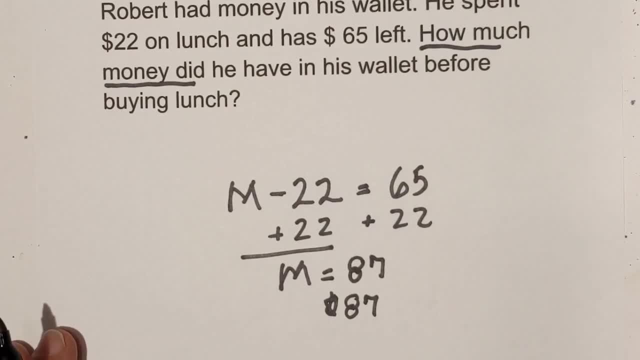 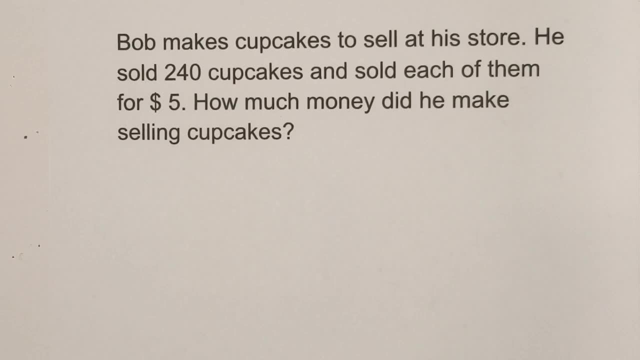 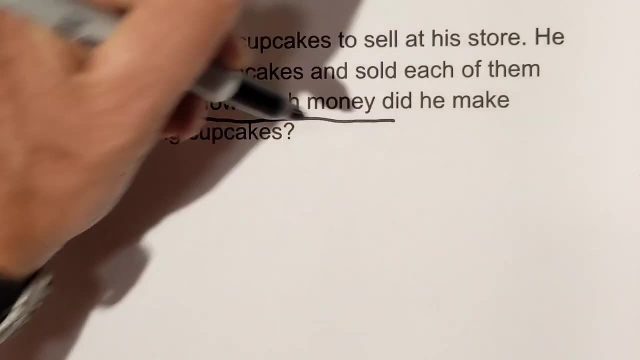 and now has $65 left in his wallet. One more, Okay. Bob makes cupcakes to sell at his store. He sold 240 cupcakes and sold each for $5.. How much money did he make selling cupcakes? Okay, The variable is how much money did he make? So let's go with again. we can go with M. 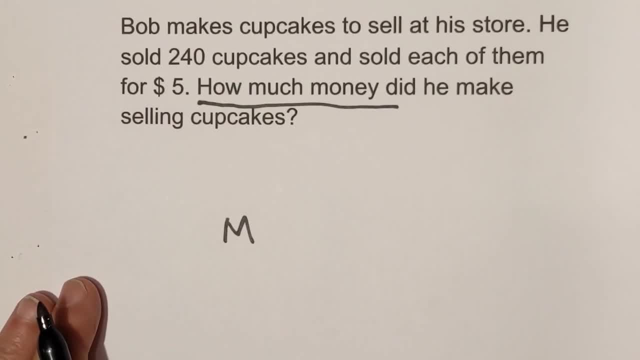 for money. Okay, I'm going to move this up a little bit, Okay, And uh, let's see what happens. We know that we want to know the grand total and he sold each. uh, sometimes that is a Q for. 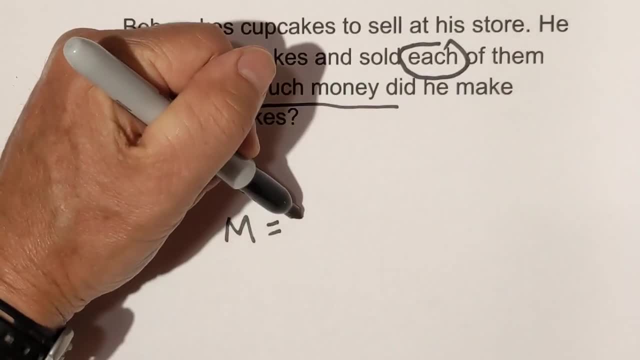 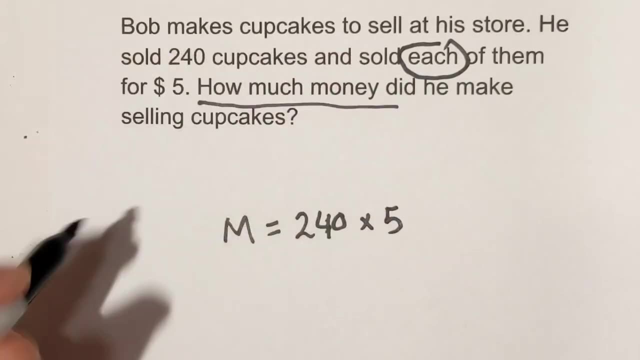 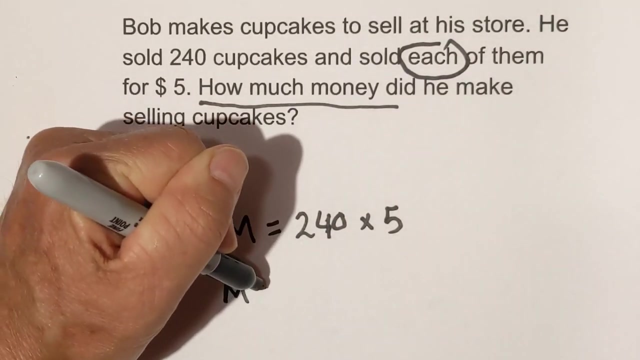 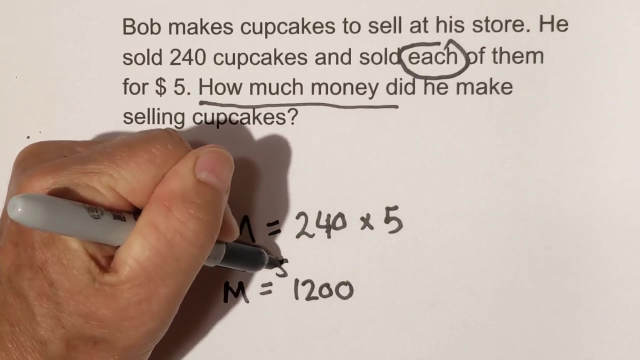 multiplication, and he sold 240, and each was $5. So M is just going to equal $2. So M is $240 times 5.. So 240 times 5 is equal to 1200, and now all we do is label it. So he made. 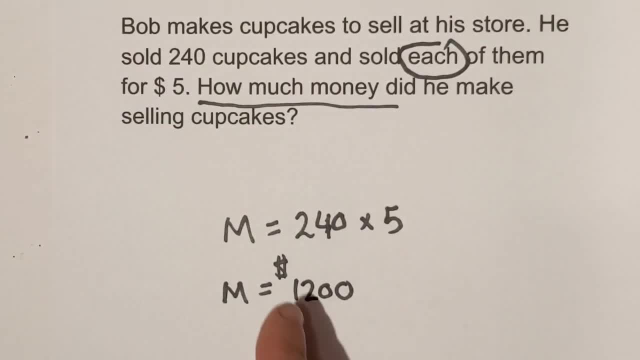 $1200, selling 240 cupcakes at $5 each. I hope this helps and remember: kindness multiplies kindness. Be kind to someone today.